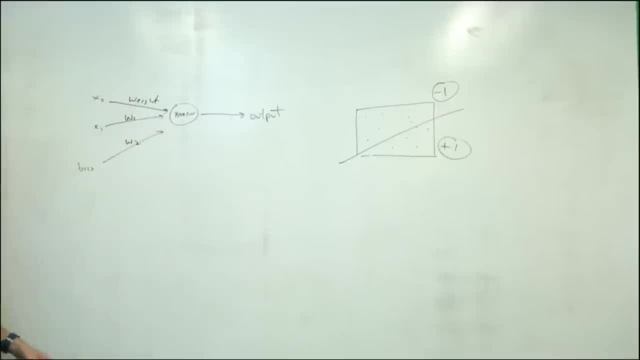 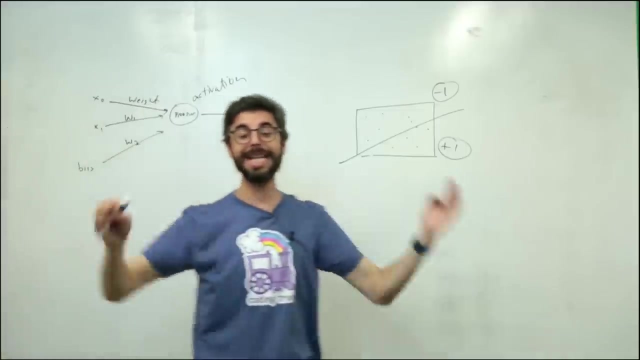 You know, weight 1,, weight 2, or whatever weight, weight, weight, And the processor creates a weighted sum of all the inputs multiplied by the weights. That weighted sum is passed through an activation function to generate the output. So why isn't this good enough? 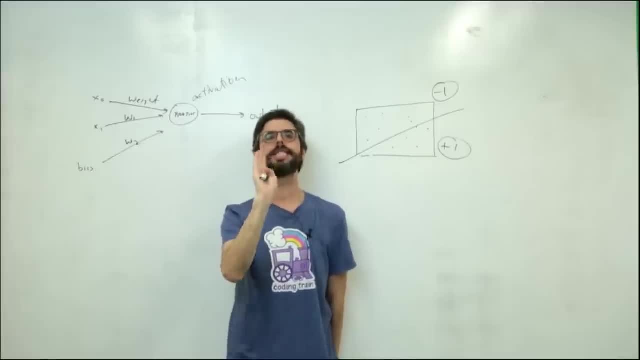 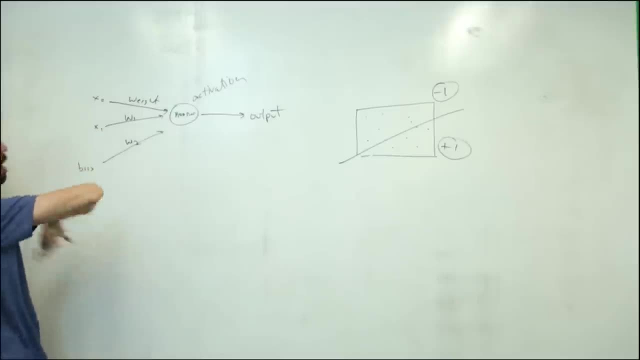 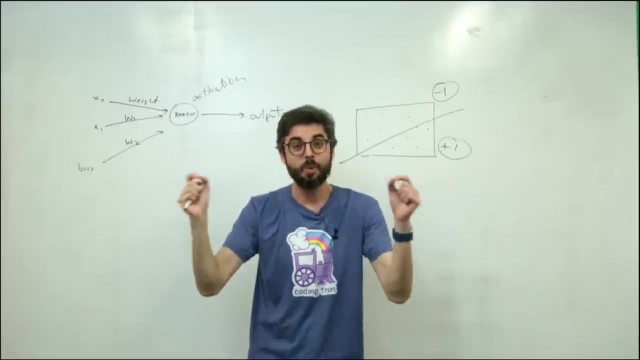 Now let's first think about what's the limit here. So the idea is that what if I want any number of inputs to generate any number of outputs? That's the essence of what I want to do in a lot of different machine learning applications. 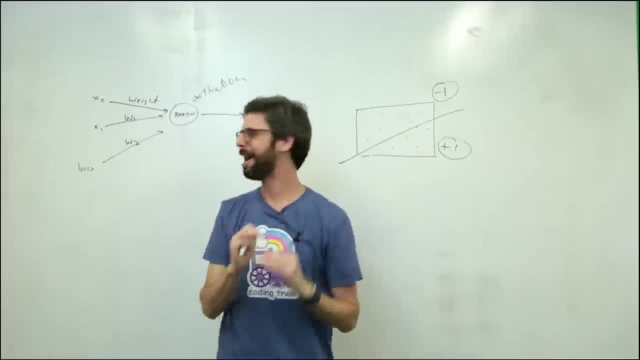 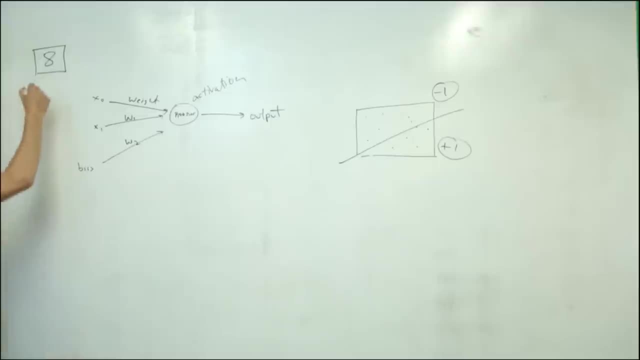 Let's take a very classic classification algorithm, which is to say: okay, well, what if I have a handwritten digit Like the number 8, and I have all of the pixels of this digit and I want those to be the inputs to this perceptron. 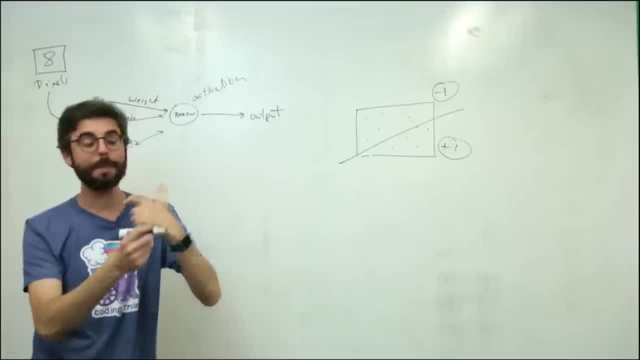 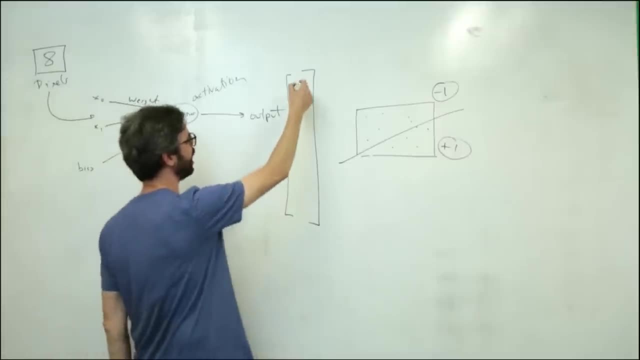 and I want the output to tell me a set of probabilities as to which digit it is. So the output should look something like: you know, there's a 0.1 chance, it's a 0,. there's a 0.2 chance, it's a 1,. 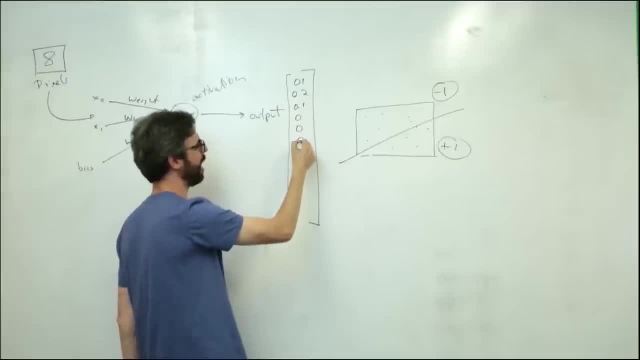 there's a 0.1 chance- it's a 2,, 0,, 3,, 4,, 5,, 6,, 7, oh, and there's like a 0.99 chance- it's an 8, and a 0.05 chance it's a 10.. 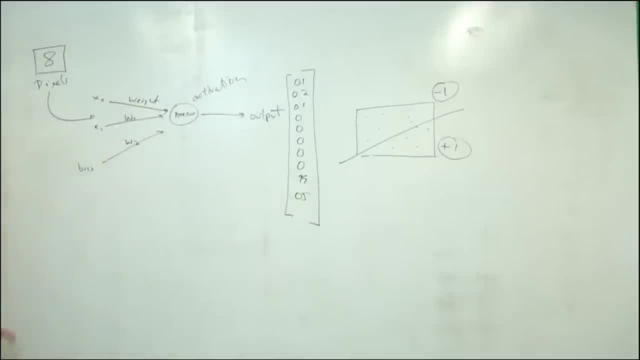 And I don't think I got those to add up to 1, but you get the idea. So the idea here is that we want to be able to have some type of processing unit that can take an arbitrary number of inputs to generate the output. 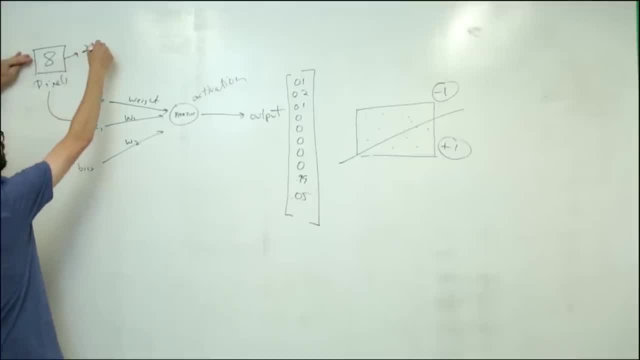 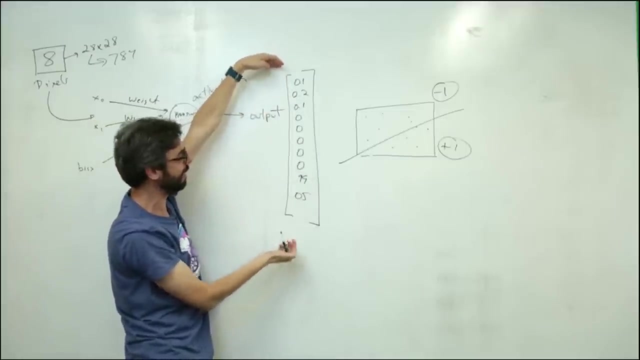 Like maybe this is a 28 by 28 pixel image, so there's 784 grayscale values and instead those are coming into the processor, which is weighted and summed and all this stuff, and we get an output that has some arbitrary amounts of probabilities to help us guess that this is an 8.. 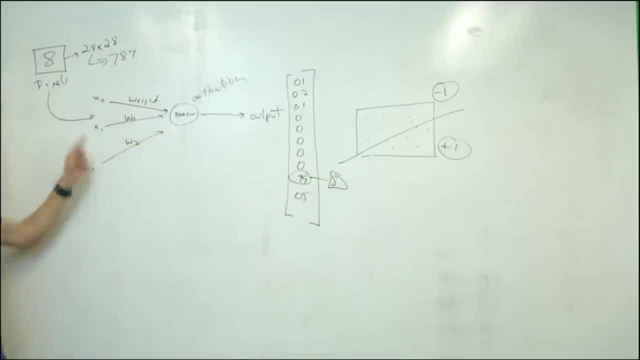 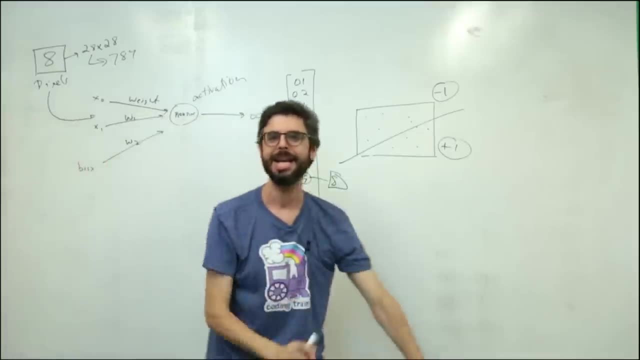 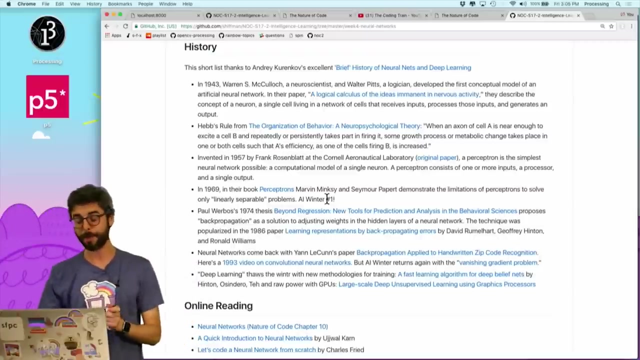 This model. why couldn't I just have a whole bunch more inputs and then a whole bunch more outputs, but still have one set of inputs, One single processing unit? And the reason why I can't is stems from an article, I don't know, sorry, a book that was published in 1969. 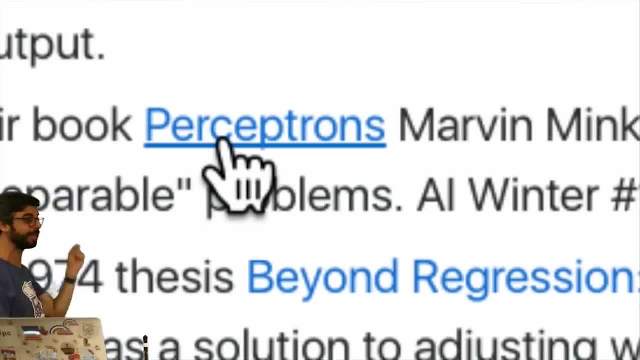 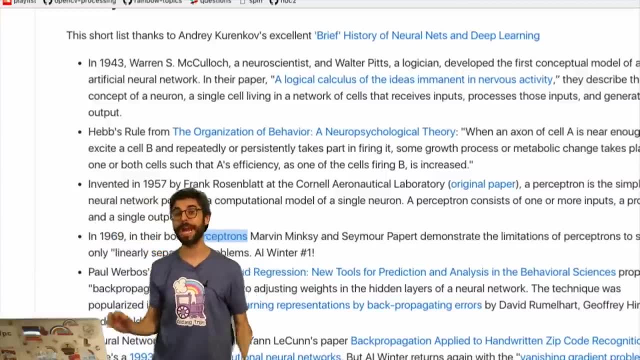 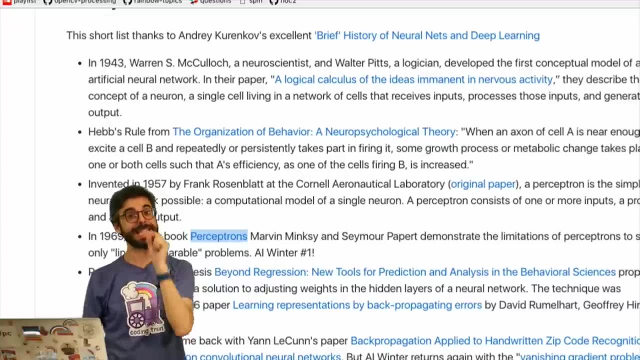 by Marvin Minsky and Seymour Papert called Perceptrons. you know AI luminaries. here In the book Perceptron, Marvin Minsky and Seymour Papert point out that a simple perceptron, the thing that I built in the previous time. 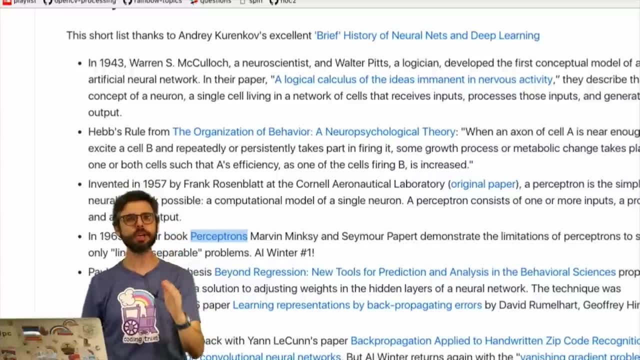 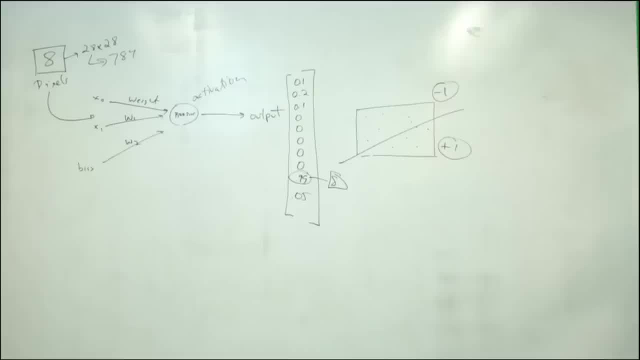 these two videos can only solve linearly separable problems. So what does that mean anyway? Why should you care about that? So let's think about this: This over here is a linearly separable problem, meaning I need to classify this stuff. 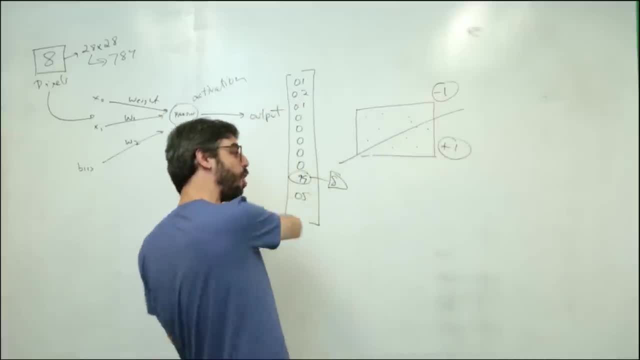 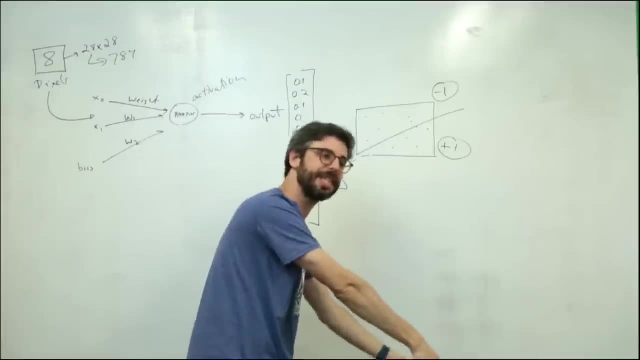 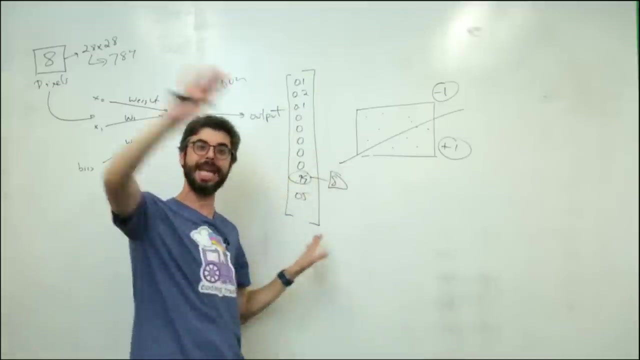 and if I were to visualize all that stuff, I can draw a line in between this part of the data, this stuff that's of this class and this stuff that's with this class. The stuff itself is separable by a line In three dimensions. I could put a plane and that would be linearly separable. 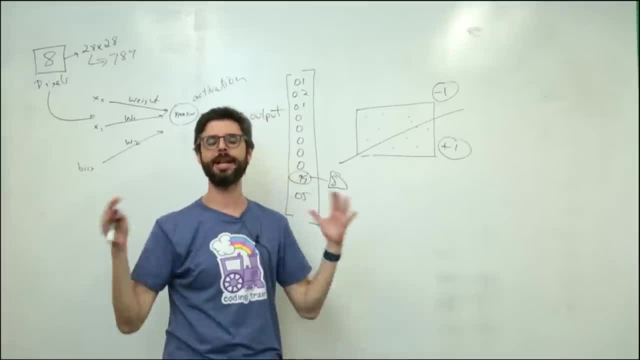 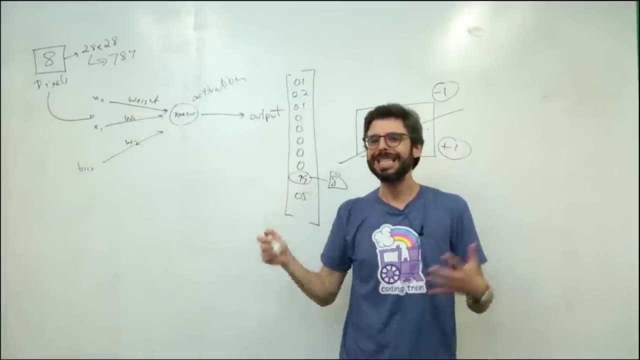 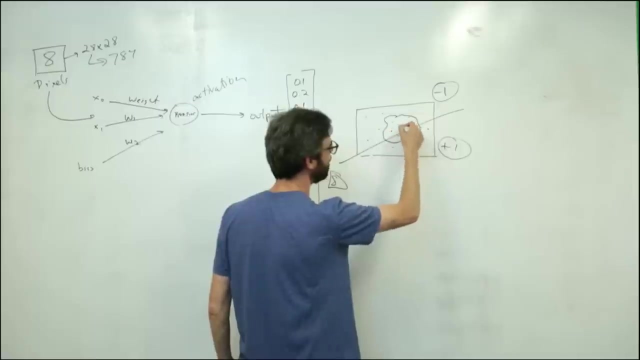 because I can kind of divide the space in half and understand it that way. The problem is most interesting. problems are not linearly separable. You know, there might be some data which clusters all here in the center. that is of one class, but anything outside of it is of another class. 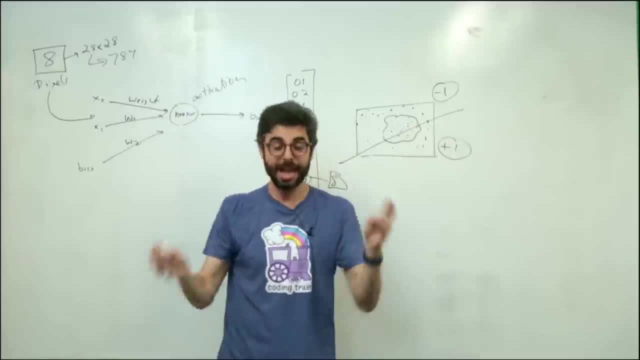 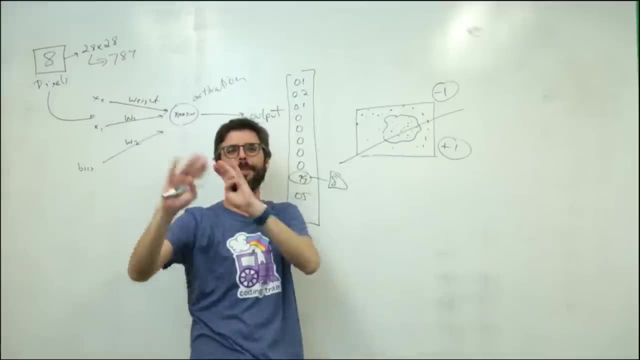 And I can't draw one line to separate that stuff. And you might be even thinking: but that's, you know still so much, You could do so much with linearly separable stuff. Well, here I'm going to show you right now a particular problem. 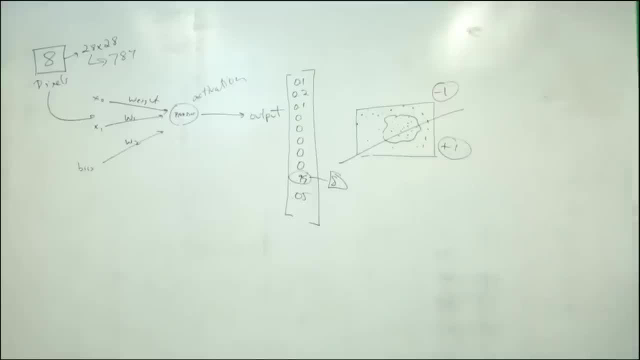 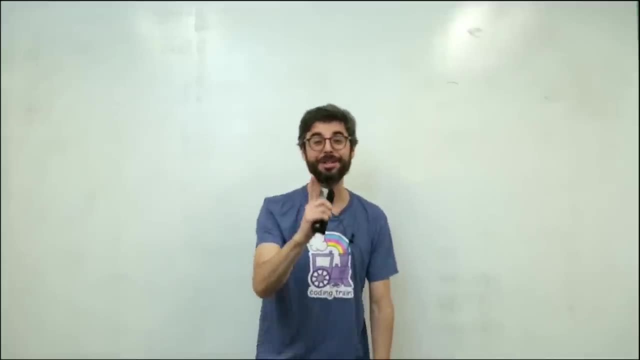 I'm looking for an eraser. I'm walking around like a crazy person. I'm going to show you a particular problem called XOR. I'm making the case for why we need to go a step further. I just had an idea. I'll come back to it later. 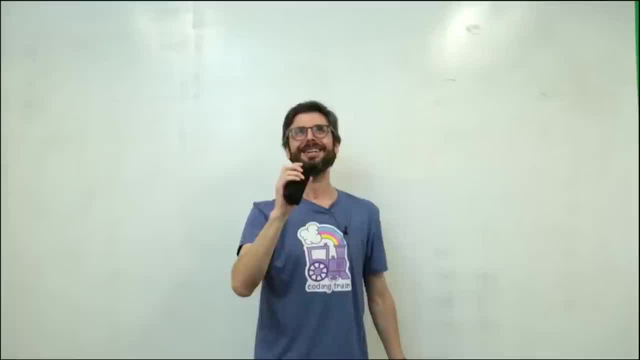 I'm making the case for why we need to go a step further and make something called a multi-layered perceptron, And I'm going to lay out that case for you right now, So you might be familiar. you might remember me from my videos. 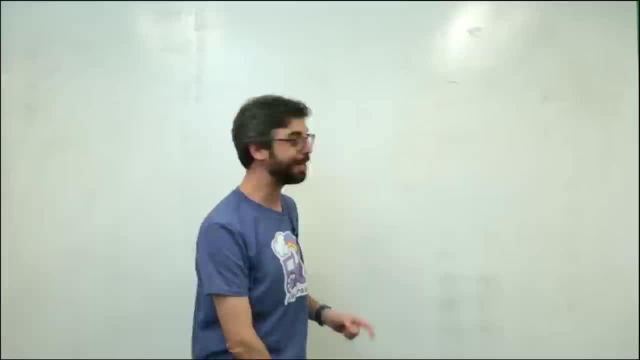 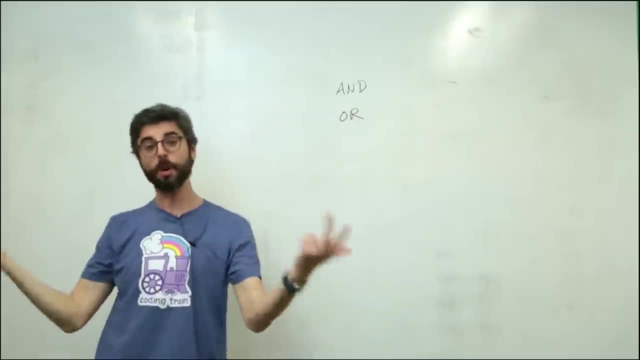 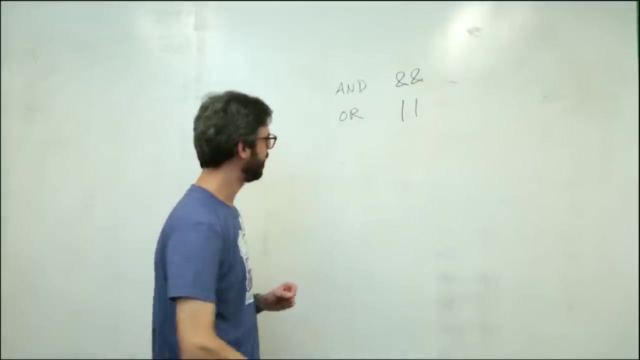 on conditional statements and Boolean expressions. Well, in those videos I talked about operations like AND and OR which, in computer programming syntax, are often written, you know, double ampersand or two pipes, The idea being that if I were to make a truth table, 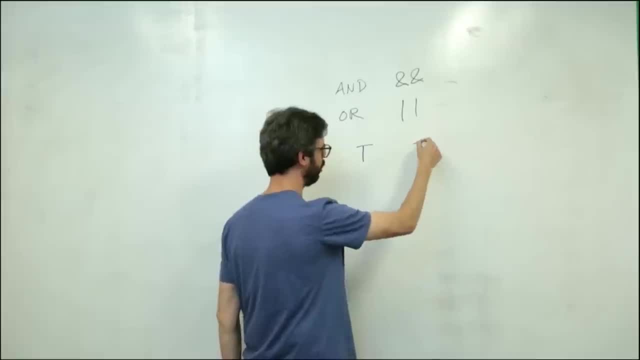 true, true, false, false. So what I'm doing now is I'm showing you a truth table. I have two elements. I'm saying: what if I say A and B? So if A is true, whoa, whoa, whoa. 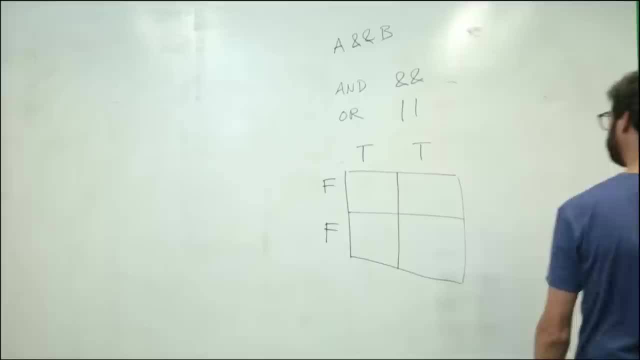 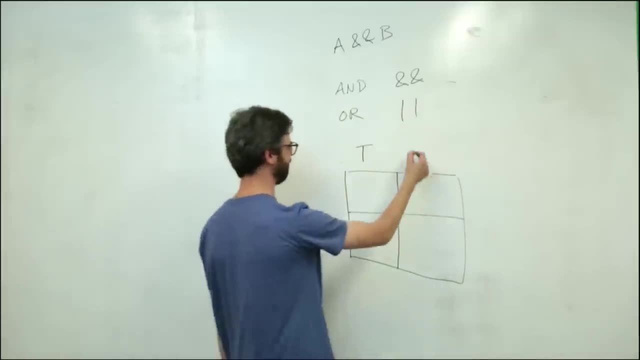 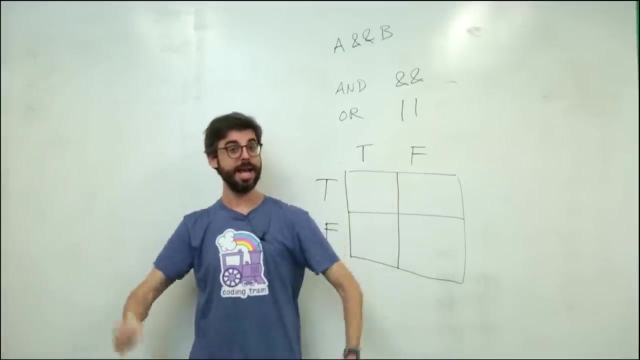 this makes no sense what I've drawn here, because I'm losing my brain cells slowly over time with every passing day. It's pretty sad. True, false, true, false, True. and true yields true If I am hungry and I am thirsty. 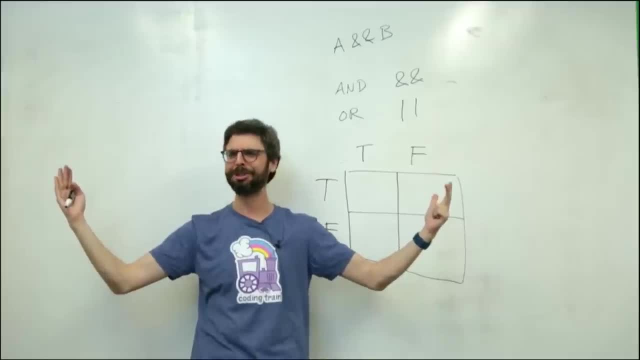 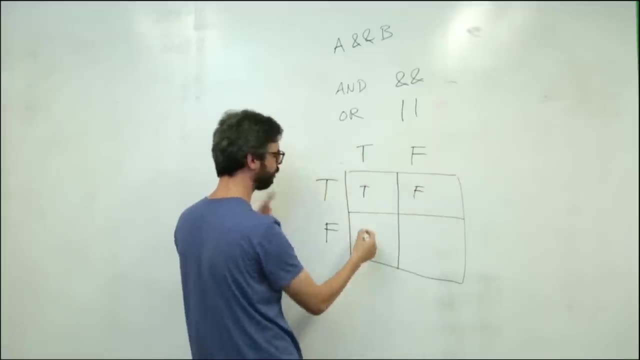 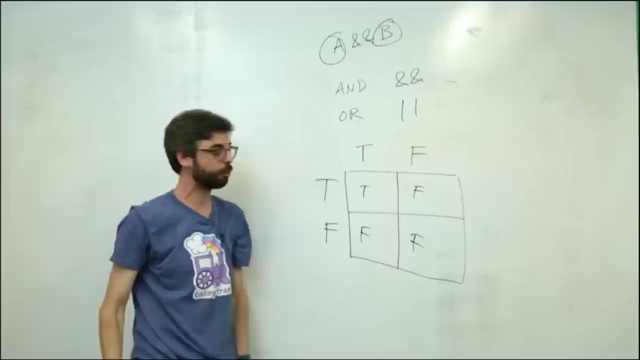 I shall go and have lunch. Right, True and true yields true. True and false is false, False and true is false, False and false is false, Right? If I have a Boolean expression A and B, I need both of those things to be true. 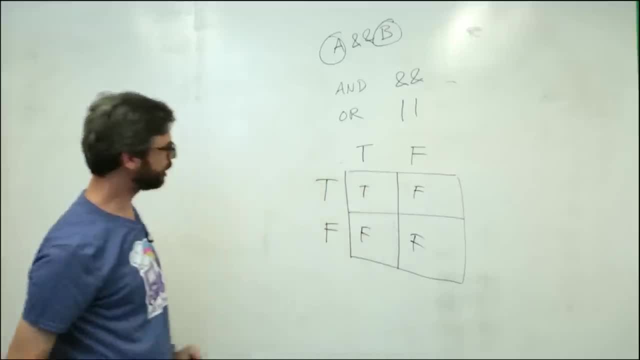 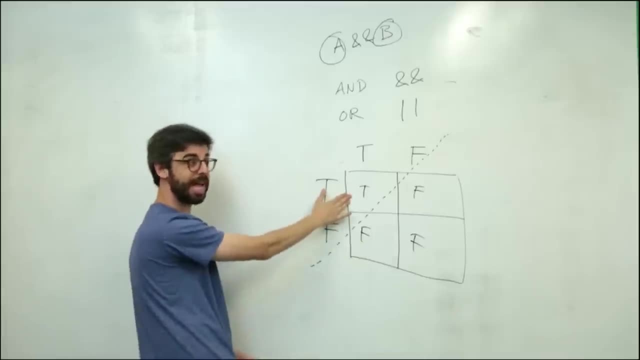 in order for me to get true. Interestingly enough, this is a linearly separable problem. I can draw a line right here and true is on one side and false is on the other side. This is a linearly separable problem. 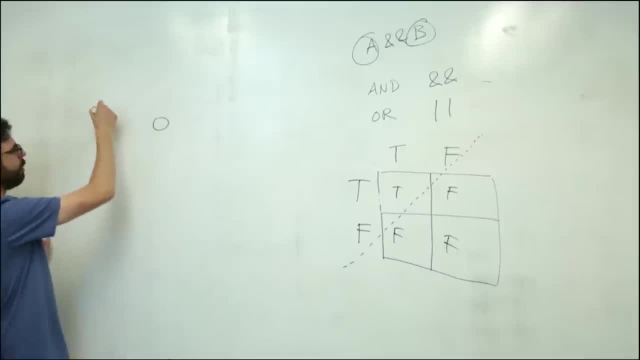 which means I could create a perceptron. That perceptron is going to have two inputs. There are going to be Boolean values- true or false, true or false- and I could train this perceptron to give me an output which, if two trues come in, 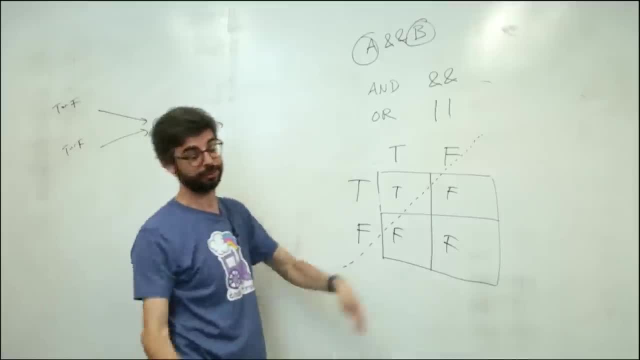 I should get a true. If one false and a true comes in, I should get a false. Two falses come in, I should get a false, Great. Or I could do the same thing. What does, or change into if I'm going to do? 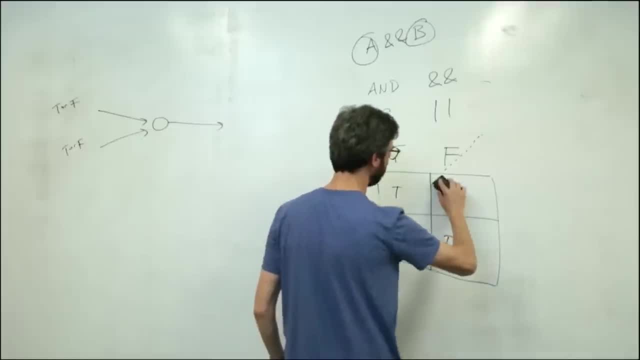 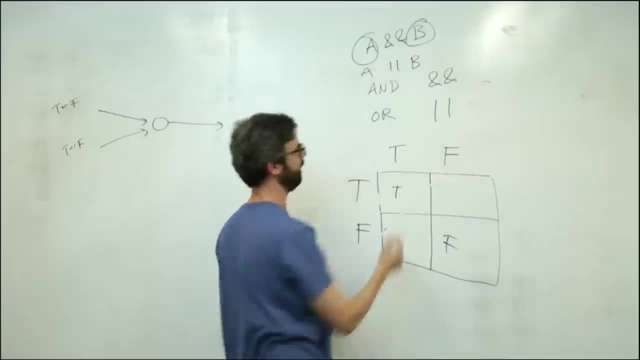 or let me erase this dotted line, and or now, ah, all of these become true, Because with an or operation A or B, I only need one of these to be true in order to get true. But if both are false, I get false. and guess what? 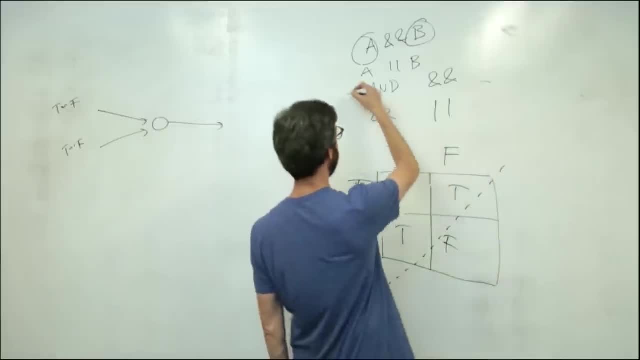 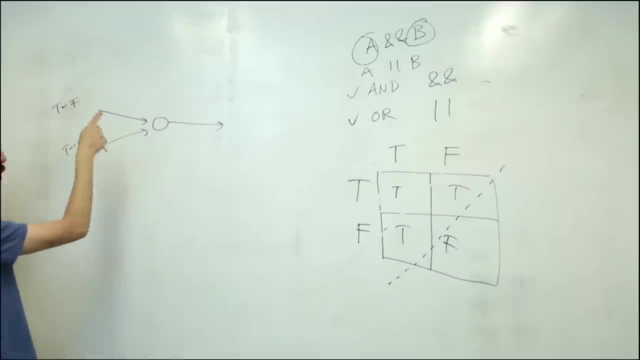 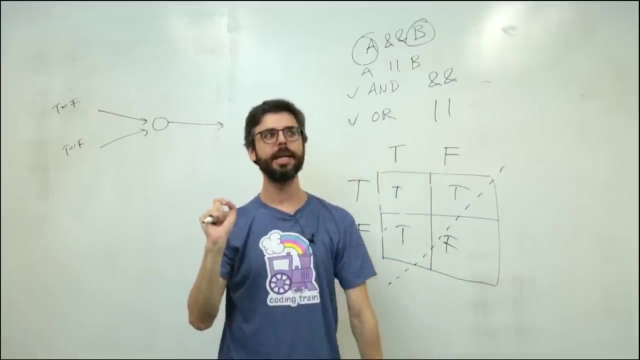 Still a linearly separable problem And is literally separable Or is literally separable. we could have a perceptron. learn to do both of those things. Now hold on a second. There is another Boolean operator which you may you might not have heard of. 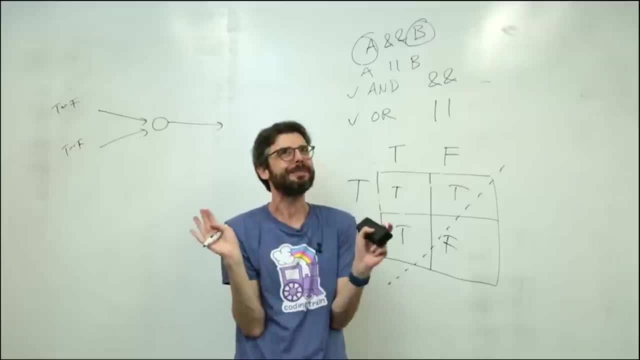 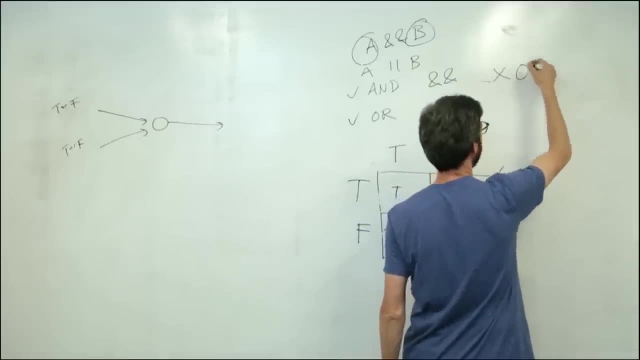 until this video, which would be really kind of exciting for me. It would make me very happy if somebody watching this has never heard of this before. It is called XOR. Can you see what I'm writing here? XOR? The X stands for exclusive. 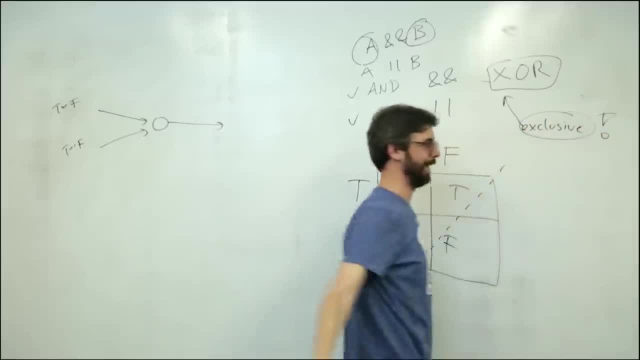 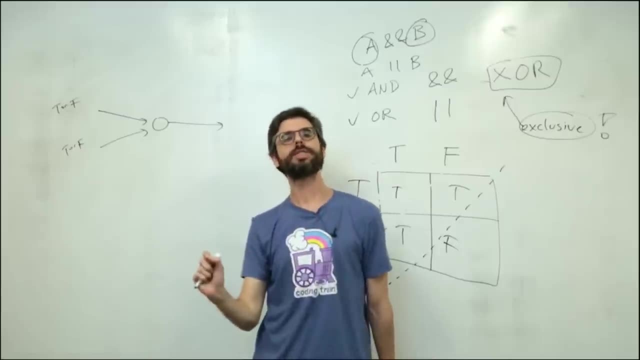 Exclusive, It's exclusive, or which means it's only true. if one is true and one is false, It's not true. both are false, this or that. if both of those things are false, I'm still false, But if both are true, it's also false. 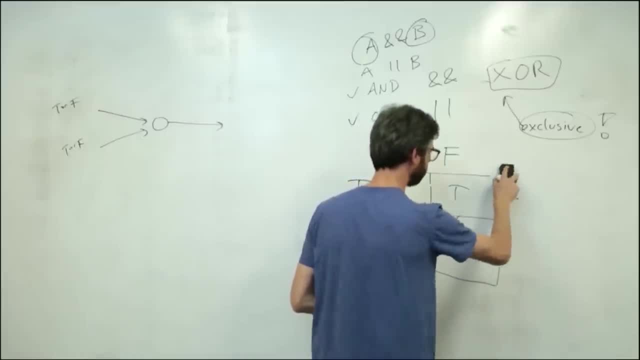 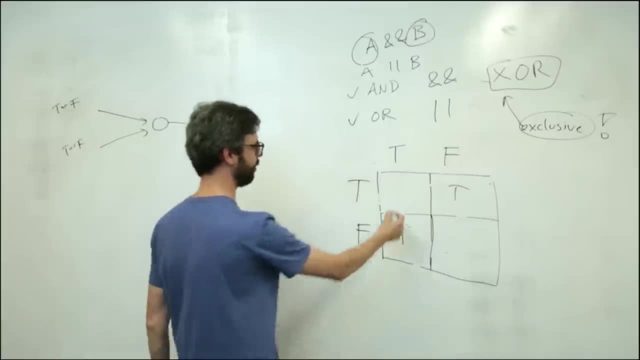 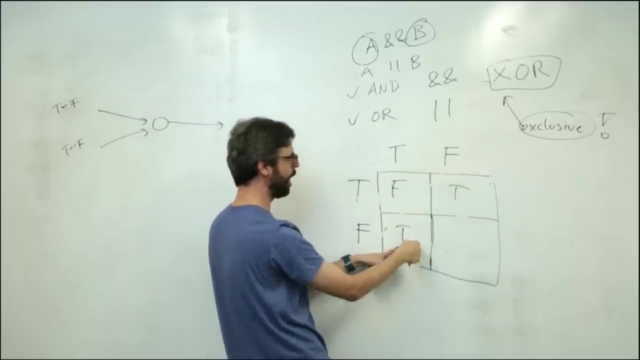 So this is exclusive, or Let me erase all this. Exclusive or means: if one is one is true and one is false, it's true. If one is true and one is false, it's true. If both are true, it's false. 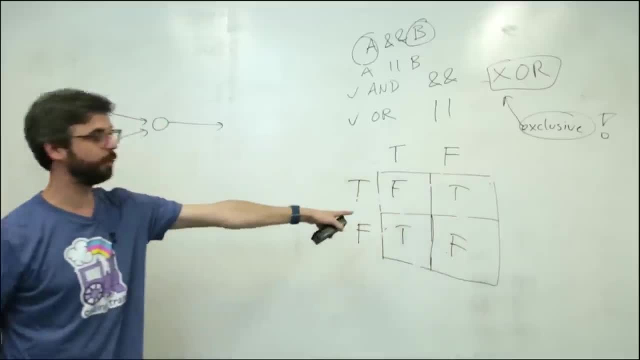 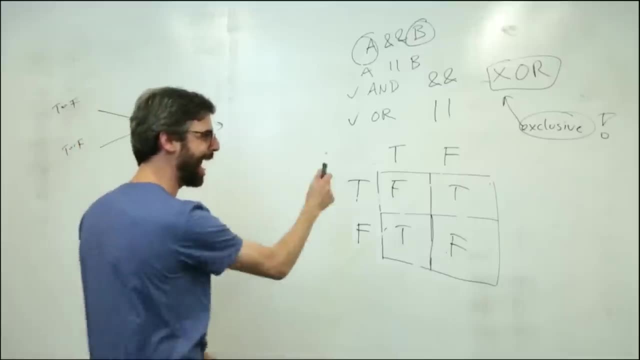 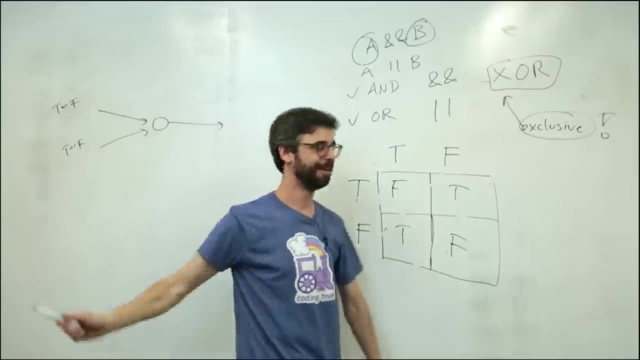 If both are false, it's false. This is exclusive or A very simple Boolean operation. However, I triple dog, dare, with the cherry on top you, to draw a single line through here to divide the falses and the trues. I cannot. 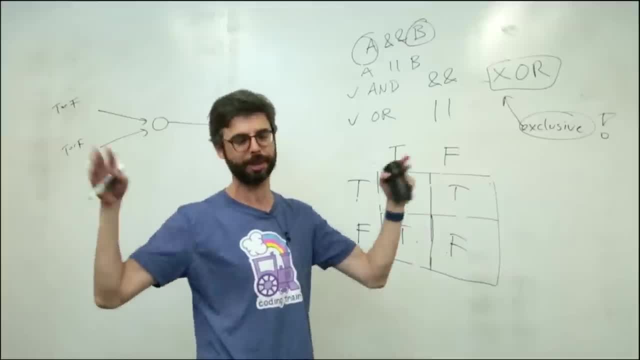 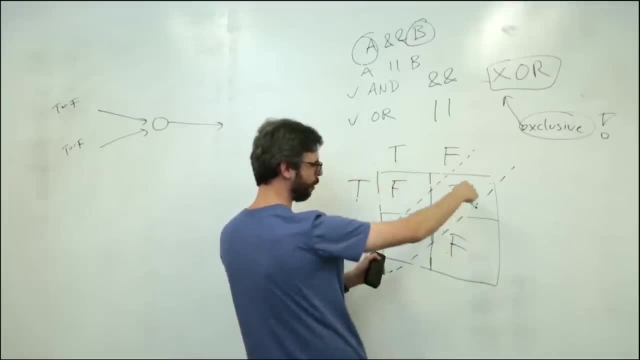 I can draw. this is not a linearly separable problem. This is the point of all this. like rambling, I could draw two lines, one here, and now I have all the trues in here and the falses outside of there. 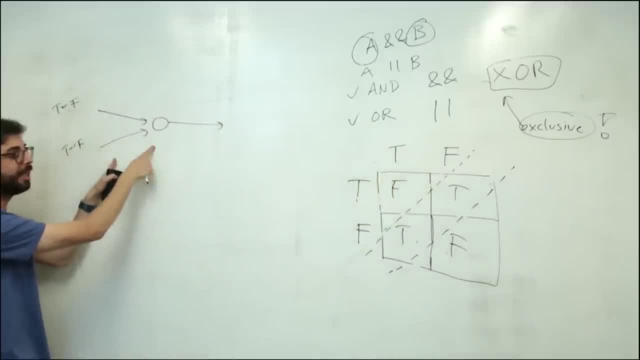 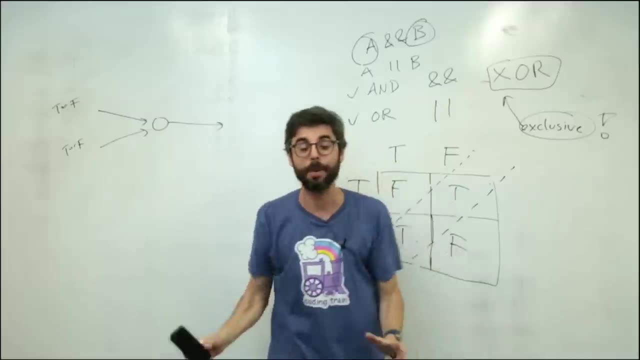 This means a single perceptron. the simplest cannot solve cannot solve a simple operation like this. So this is what Minsky and Papert talked about in the book: perceptrons. Well, this is like an interesting idea conceptually. 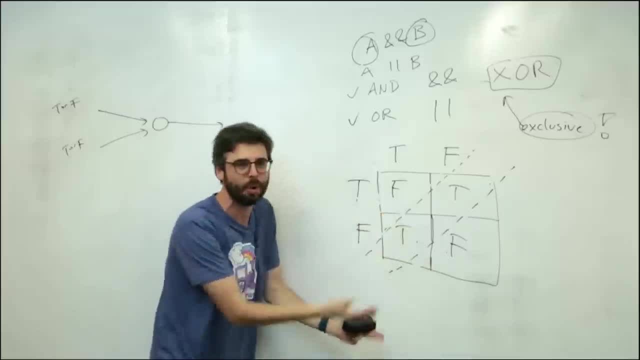 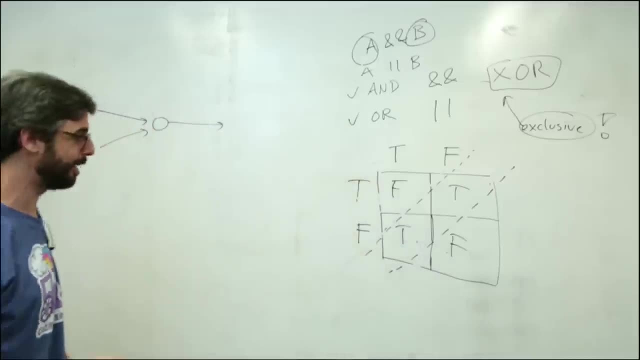 It kind of seems very exciting, but if it can't solve XOR, what are we supposed to do with this? The answer to this is- and you might have already thought of this yourself- it's not too much. I kind of missed a little piece of my diagram here. 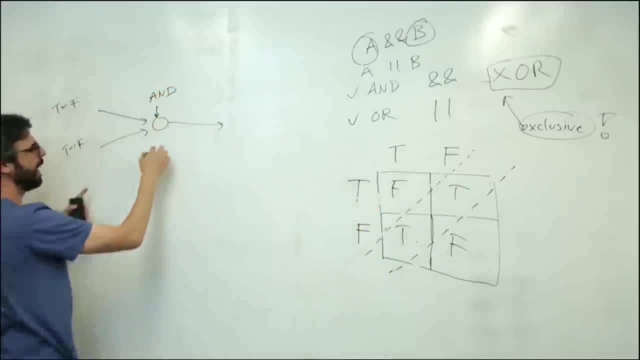 Let's say, this is a perceptron that knows how to solve, AND And this is a perceptron that knows how to solve, OR What if I took those same inputs and sent them into both And then I got the output here? So this output. 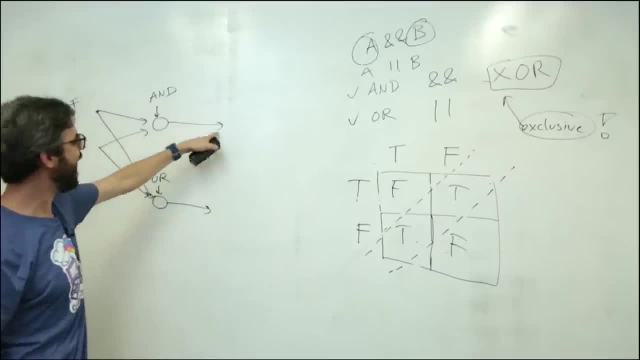 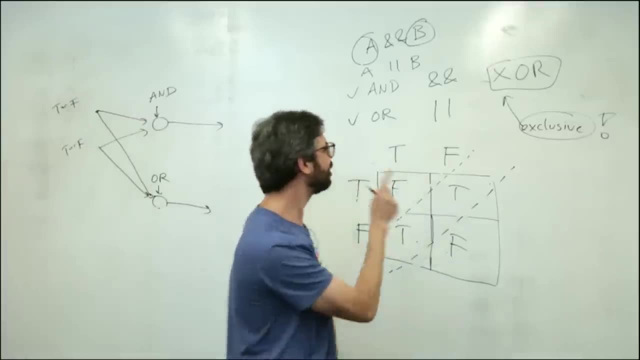 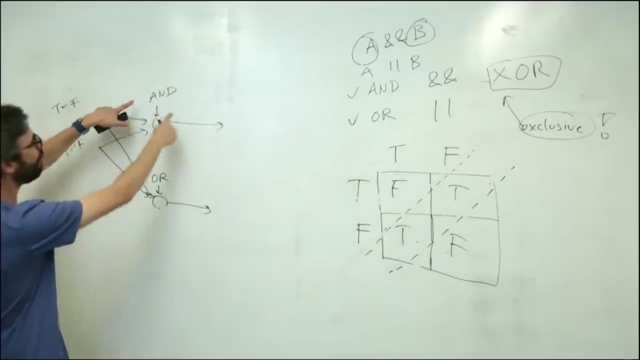 would give me the result of AND, and this output would give me the result of OR. Well, what is XOR really? XOR is actually OR, but not AND. Right? So if I can solve something, AND is linearly separable. 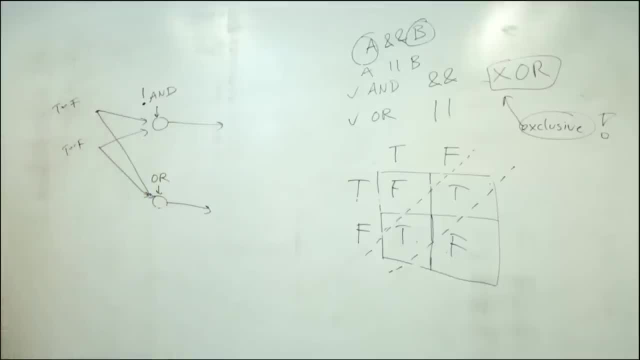 NOT AND is also linearly separable. So what I want, then, is for both of these outputs actually to go into another perceptron. that would then be AND. So if this perceptron can solve NOT AND, and this perceptron can solve OR, 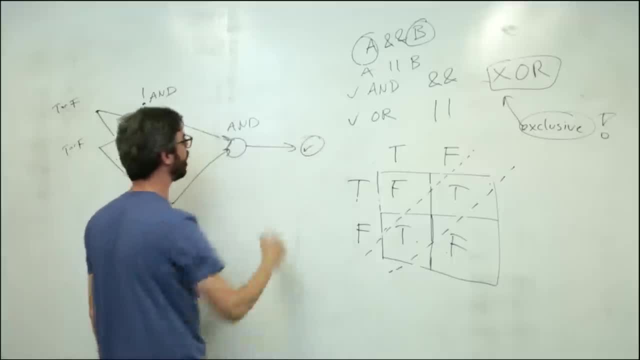 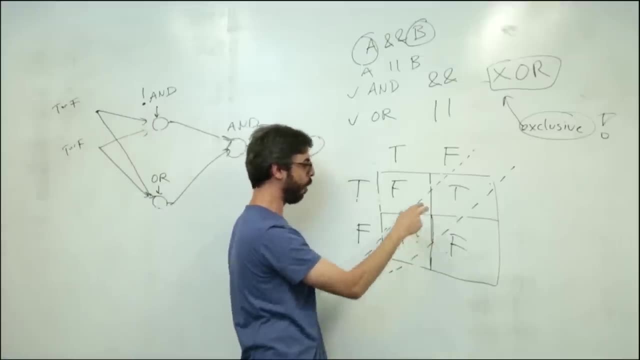 and those outputs can come into here, then this would be the result of both: OR is true and NOT AND is true, Which is actually this: These are the only two things where OR is true but NOT AND, And so the idea here is that. 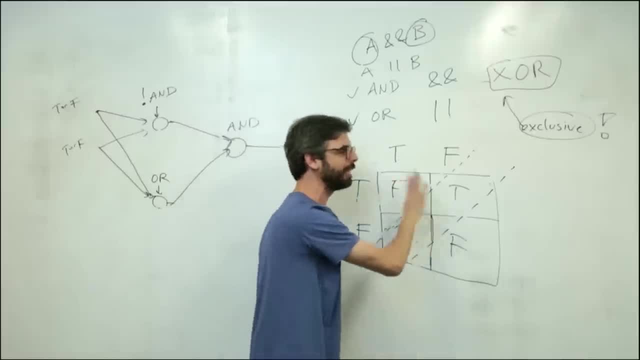 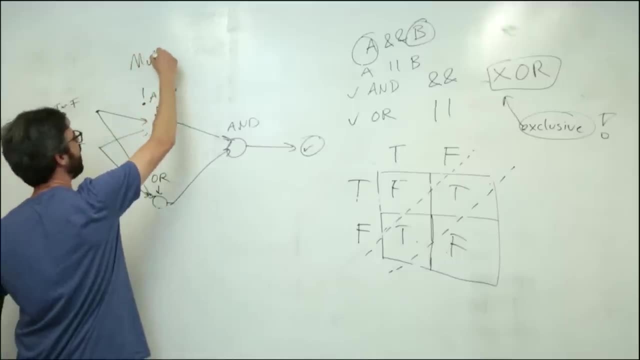 more complex problems that are not linearly separable can be solved by linking multiple perceptrons together, And this is the idea of a multi-layered perceptron. We have multiple layers, and this is still a very simple diagram. You could think of this almost as like. 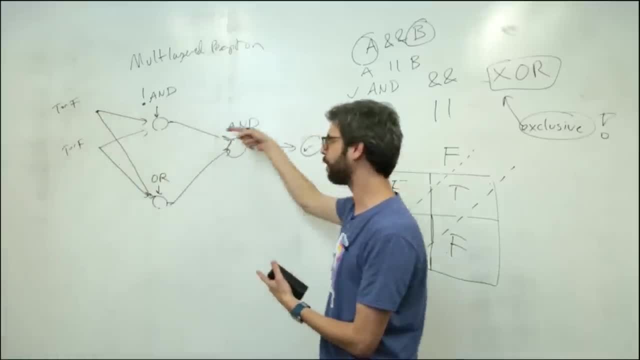 if you were designing a circuit right, If you decide whether electricity should flow- and this were like a, these were switches- you know how could you get a bunch of, how could you have an LED turn on with exclusive, OR You would actually wire the circuit. 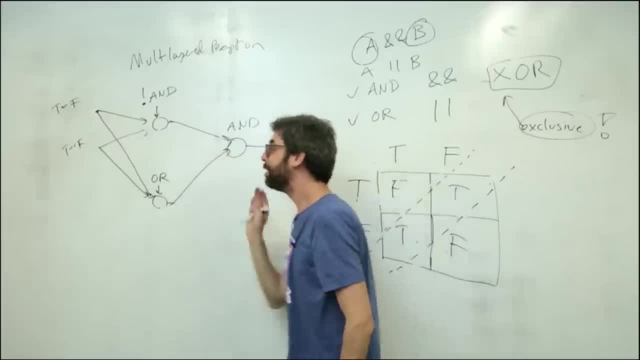 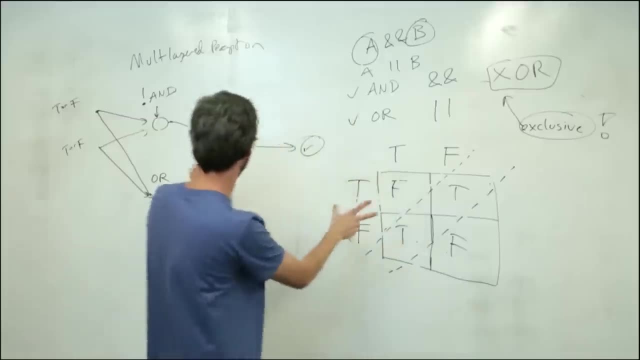 basically in exactly this way. So this is the idea here. So what I would like to do in the next. so at some point I would like to make a video where I actually just kind of build, take that previous perceptron example and just take it a few steps farther. 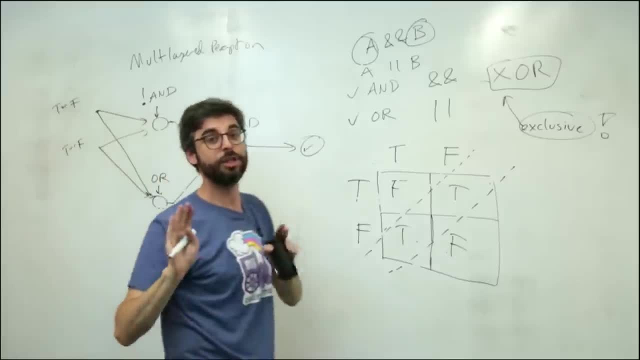 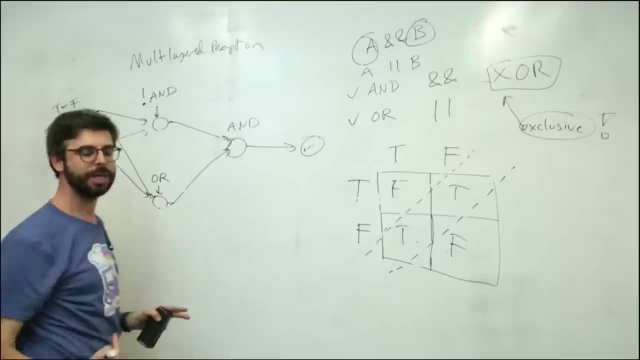 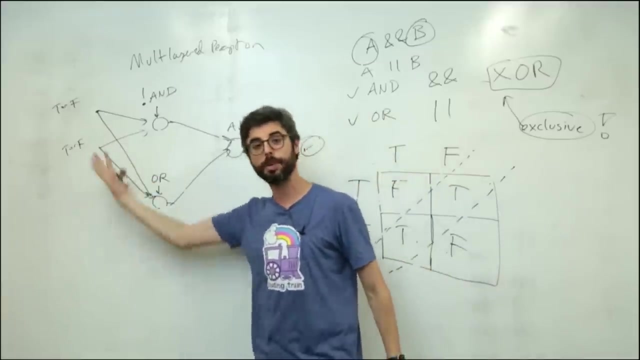 to do exactly this. But what I'm going to do actually in the next video is diagram out this structure of a multi-layered perceptron, how the inputs, how the outputs work, how the feed-forward algorithm works. where the inputs come in get multiplied by weights. 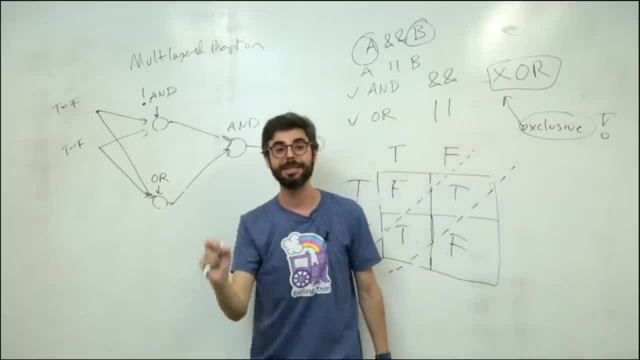 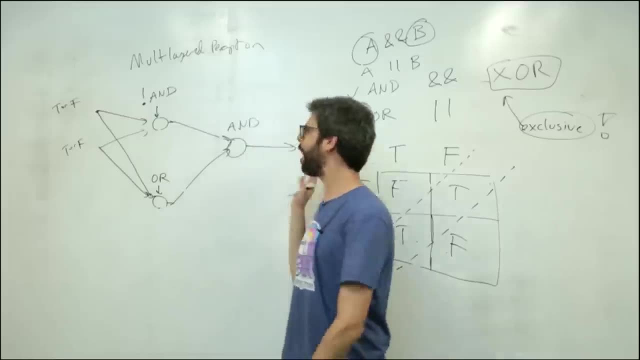 get summed together and generate an output and build a simple JavaScript library that has all the pieces of that neural network system in it. Okay, So I hope that this video kind of gives you a nice follow-up from the perceptron and a sense of why. 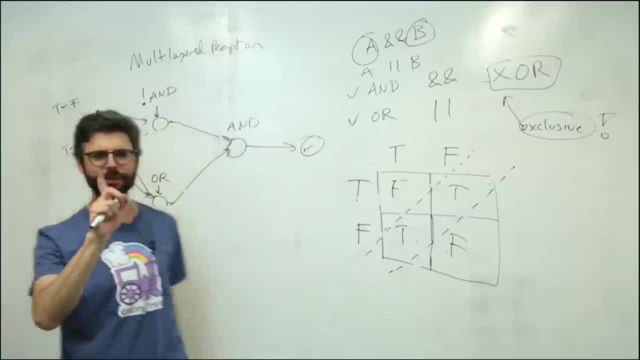 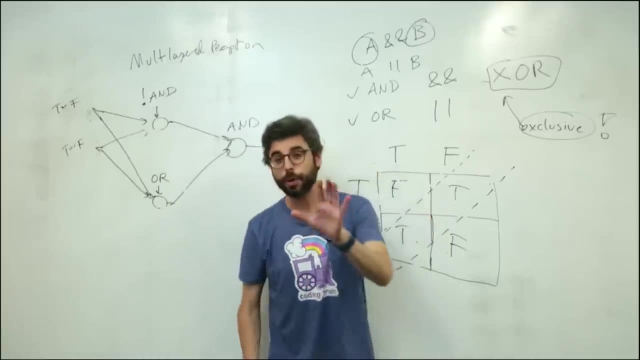 this is important And I'm not sure if I'm done yet. I'm going to go check the live chat and see if there are any questions or important things that I missed, and then this video will be over. Okay, I'm back. So there was one question. 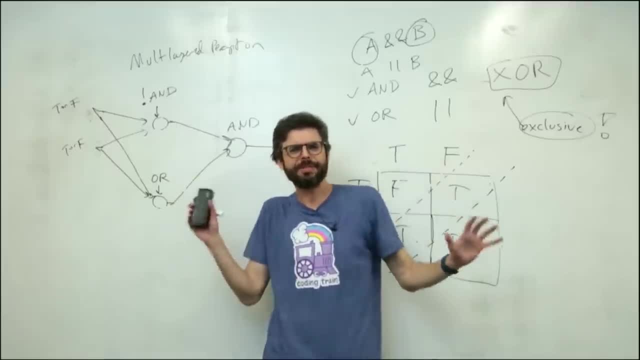 which is important, like oh what? I heard somebody in the chat ask: what about the hidden layer? And so this is jumping ahead a little bit, because I'm going to get to this in more detail in the next video- The way that I drew this diagram. 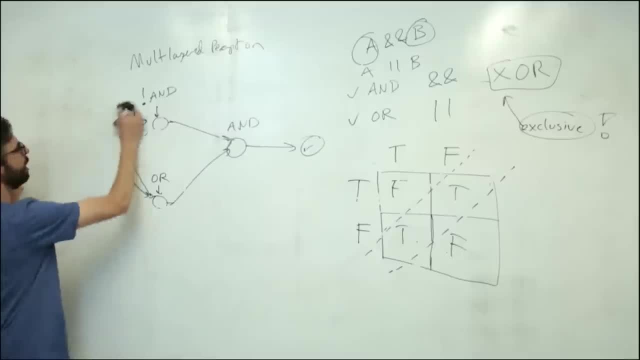 is pretty awkward. Let me try to fix this up for a second. Imagine: there were two inputs and I actually drew those as if they were neurons- and I know I'm out of the frame, but I'm still here- And these inputs were connected to each of these perceptrons. 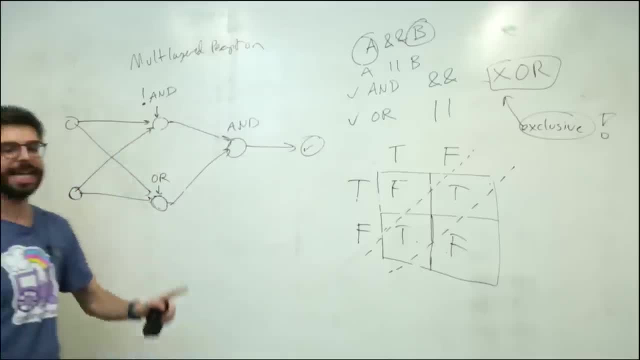 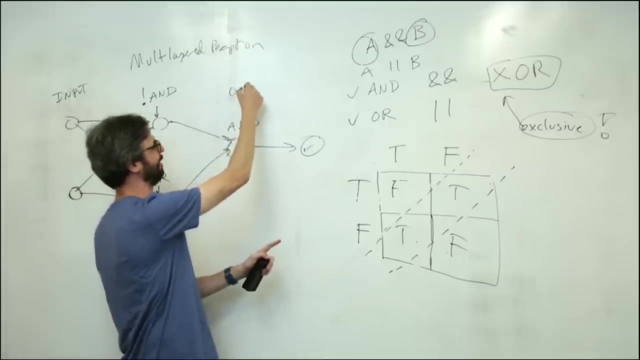 Each was connected and each was weighted, So this is actually what's now known as a three layer network. There is the input layer. This is the hidden layer and the reason why it's okay. well, actually this is the output layer. That's obvious, right? 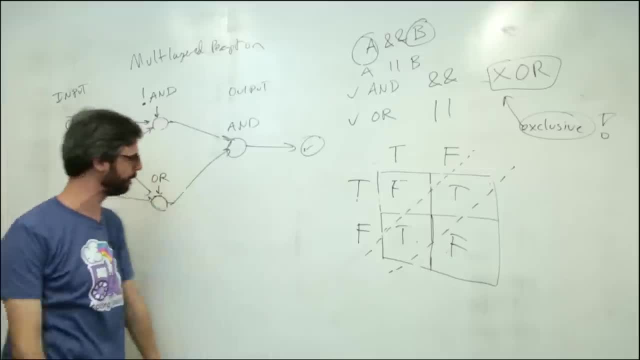 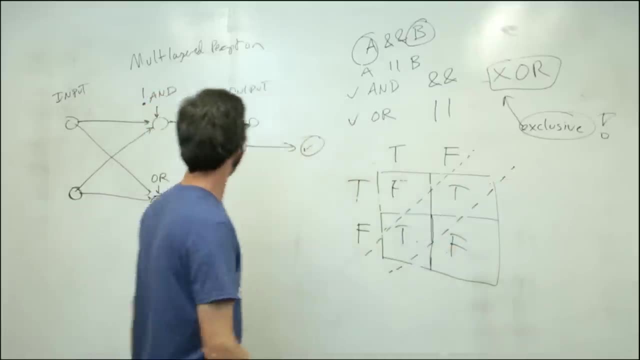 This is the input. Those are the inputs, the trues and the falses. This is the output layer that should give us a result: Are we still true or are we false? And then the hidden layer are the neurons that sit in between the inputs and the outputs. 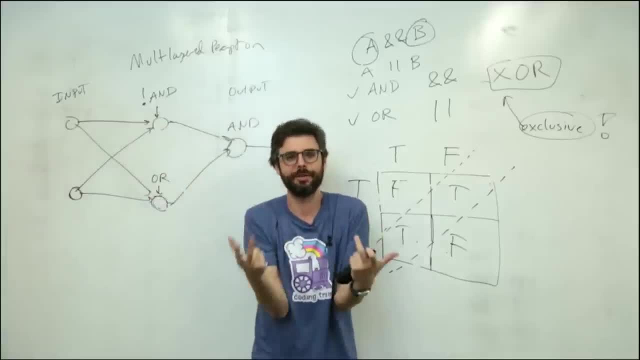 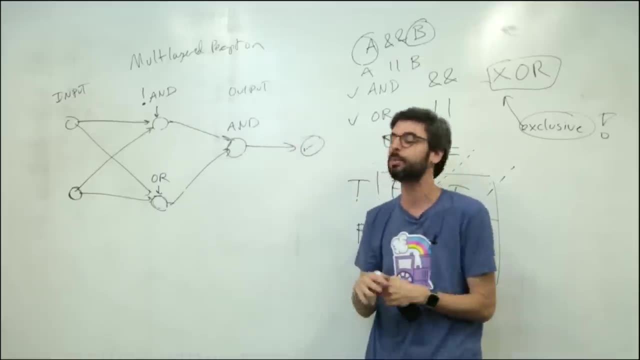 and they're called hidden because, as a kind of user of the system, we don't necessarily see them. A user of the system is feeding in data and looking at the output. The hidden layer, in a sense, is where the magic happens. The hidden layer.